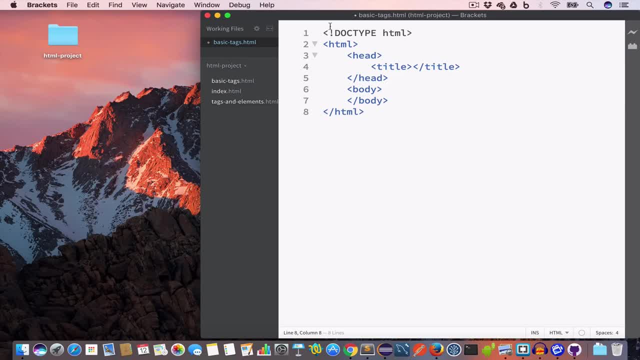 and we'll write the basic HTML. So we have the doc type HTML. opening and closing HTML tag. opening and closing head tag and inside this we have the title tag. We'll set the title to basic tags and we have the opening and closing body tag. Now let us open the. 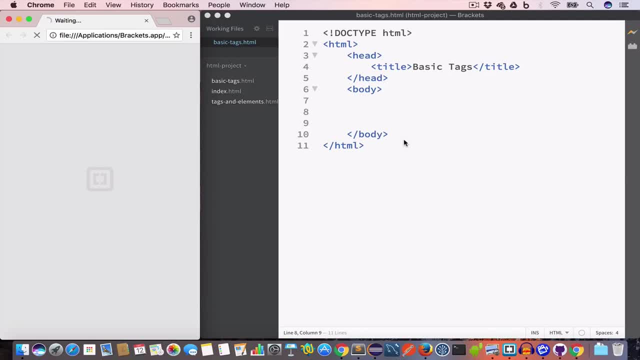 live preview. We'll begin our journey by first creating heading tags. Now, in HTML, there are six different types of heading tags: H1, H2, H3 till H6. And in most of the cases, you will need H1, H2 and H3.. So let's create the heading tags. 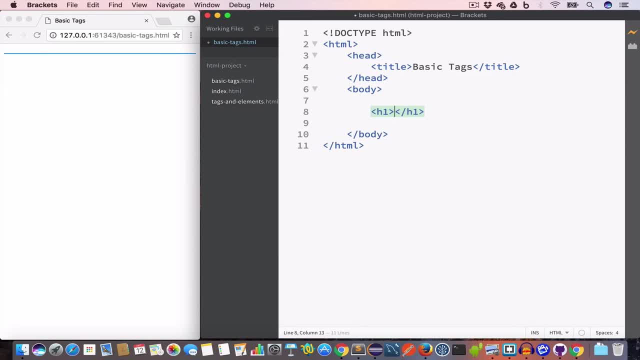 So the first example is H1. So we will write heading H1.. Similarly, you can create H2 tags having second priority, so h1 having the highest priority, then h2, and if you want, you can also create h3 tags, heading h3, and similarly h4 tags. 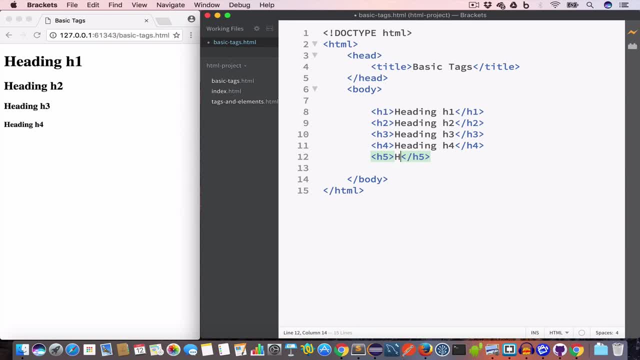 h5 tags and h6 tags and if you look at the output you can see h1 tag has a bigger font and h6 heading tag is of smaller font. the heading tags are block elements, that is, they take up the entire width and they have a new line before. 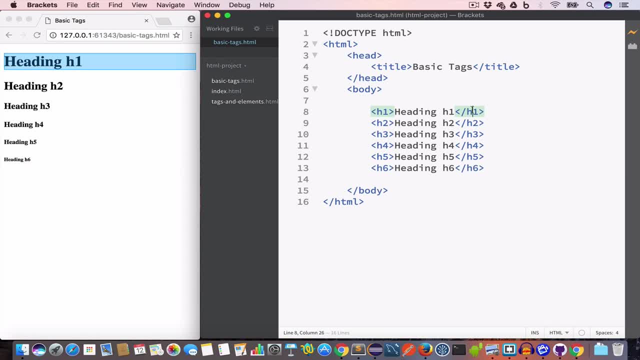 and after them. so if you consider h1 tag, you can see it takes up the entire width. similarly h2 tag, h3 tag, 4, 5 and 6. the next tag that we are going to talk about is the paragraph tag and, as the name suggests, it is: 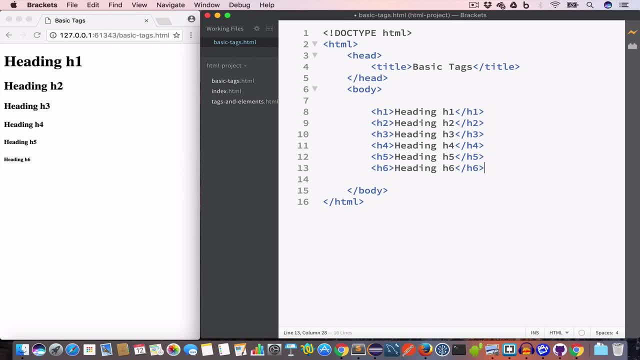 used to create paragraphs. so to create a paragraph tag, we use the p character and we can write: this is a sample paragraph. a paragraph tag is also a block element. so if we create a new paragraph- this is the second para you can see- it takes a new line and occupies the entire width. 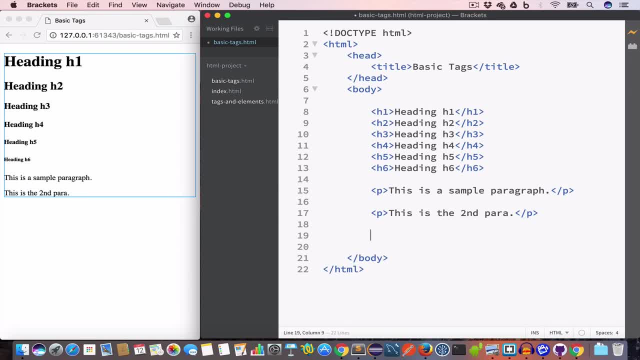 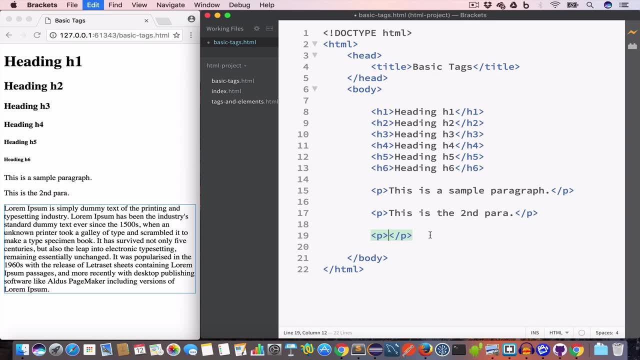 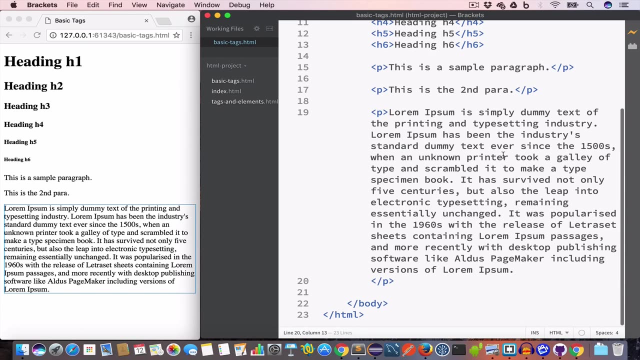 similarly, we can create another paragraph and write some random text like so, and you can see, this new paragraph is taking the entire width and since it's a block element, so it is starting from a new line. this is a block element, so it is starting from a new line. 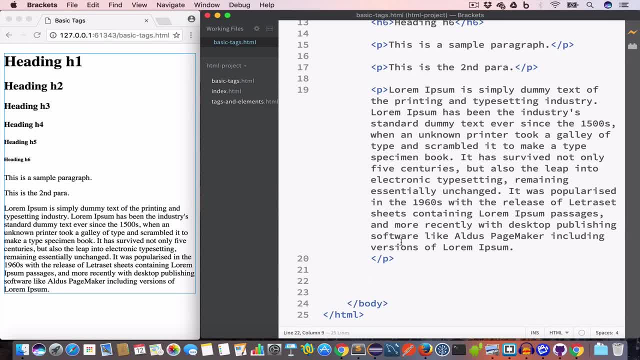 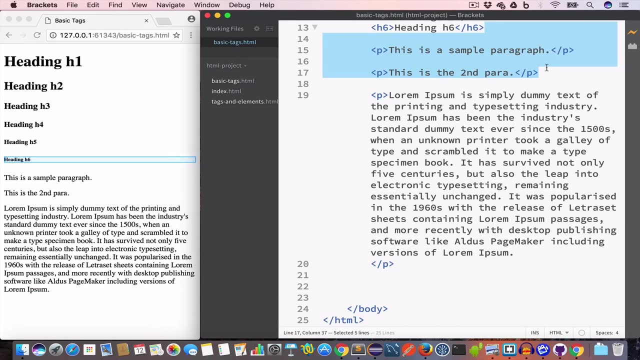 the next tag is used to create horizontal line and it is called the hr tag. so let's say we have two paragraphs and we want to create a horizontal line between the two. we'll use the hr tag. Let me go ahead and copy this. So let's say we have two paragraphs. 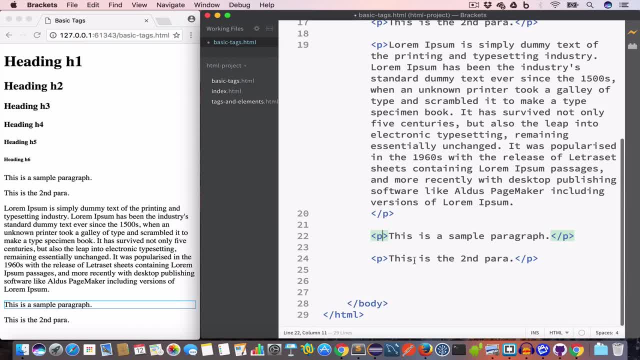 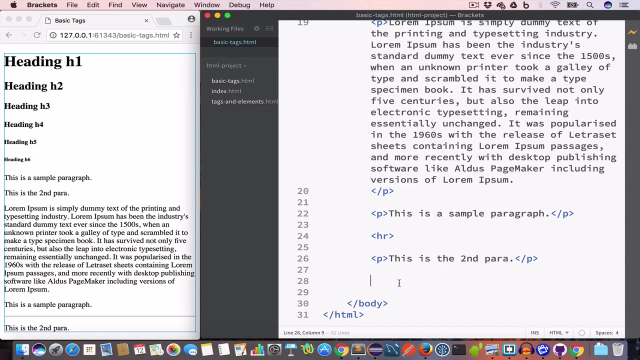 This is a sample paragraph and we have another paragraph- This is the second paragraph- and we want a horizontal line, So we'll create the HR tag And you can see we have a horizontal line between the two paragraphs. The next tag is the line break tag or the BR tag. 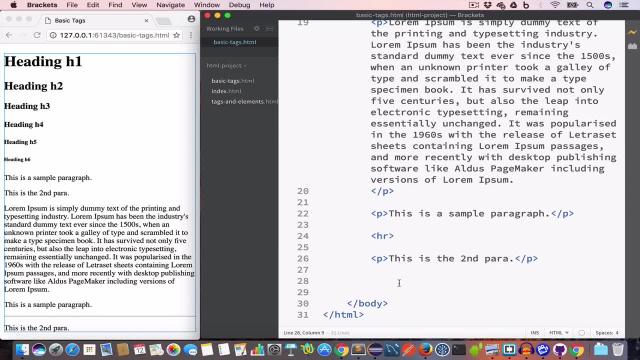 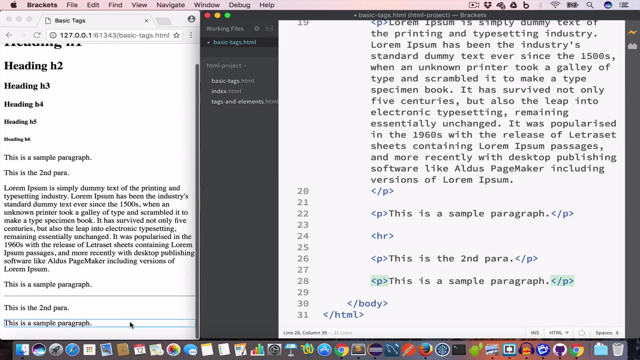 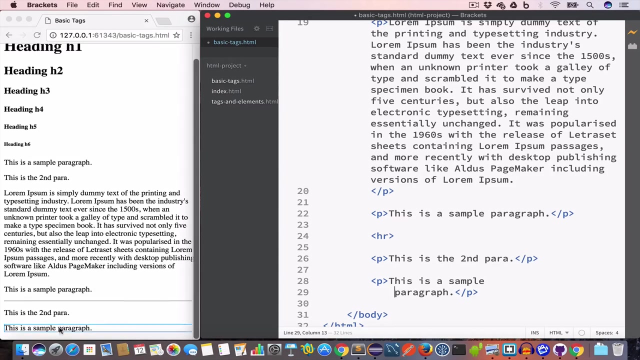 It is used to make any content after the BR tag start from a new line. So, for example, let's say we create a paragraph. This is a sample paragraph. So you can see we have the output. This is a sample paragraph. Now if we move this paragraph word to the next line, we can see we still have the same. 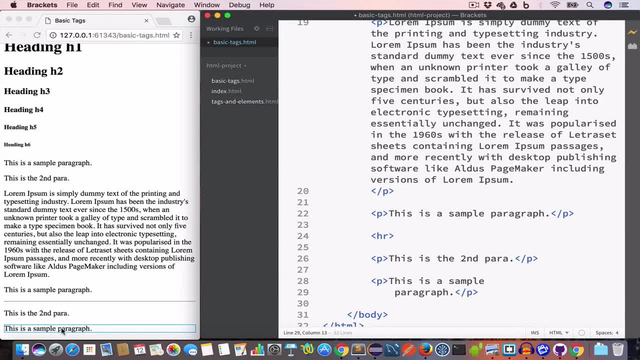 output and this paragraph word is still at the same line. Now, in order to move this paragraph word to the next line, we use the BR tag, Because in HTML, even if you add multiple white spaces, HTML will still count them as one space. 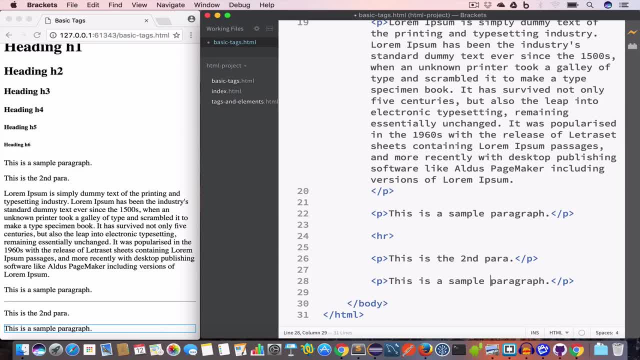 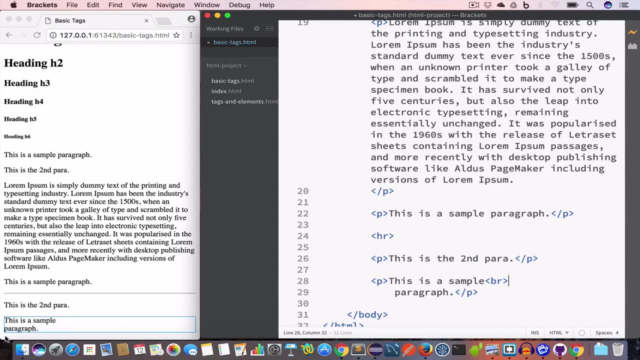 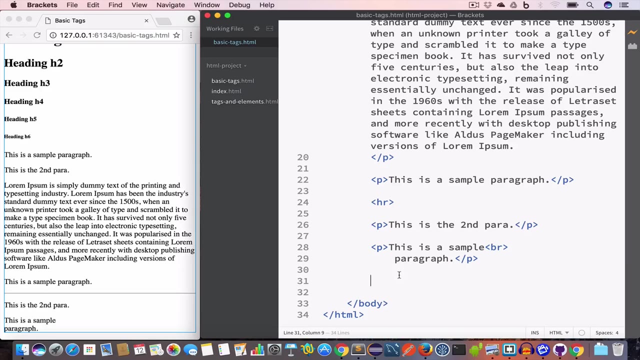 So, in order to make this paragraph word appear at the next line, we use the BR tag, And now you can see the word. paragraph starts at the next line. The next tag that we're going to talk about is called the code tag. It is used to display code in our web page. 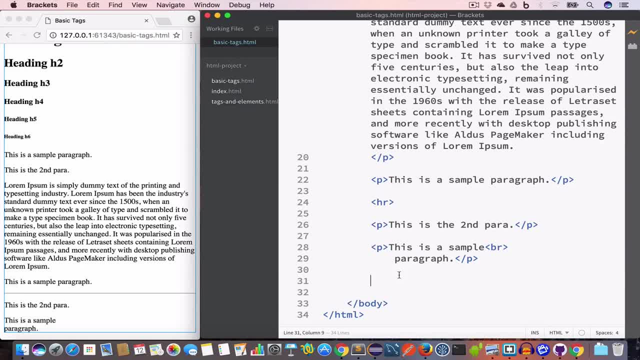 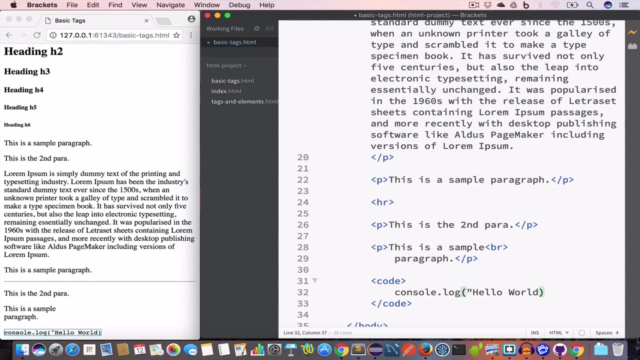 So let's say we want to display a JavaScript code in our web page, So we'll write code And inside this we can write, let's say, consolelog, Hello world. So you can see, we have this output: consolelog- hello world. 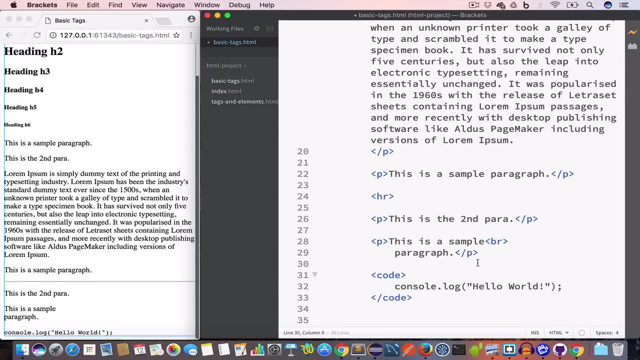 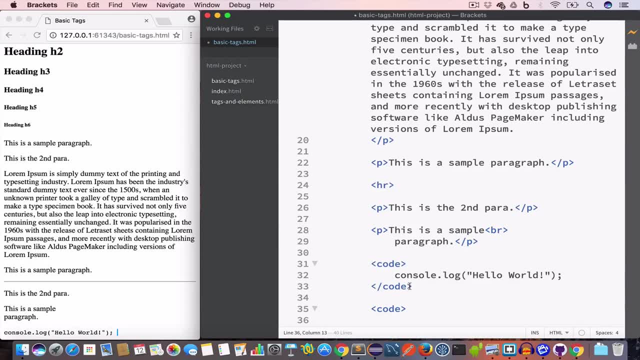 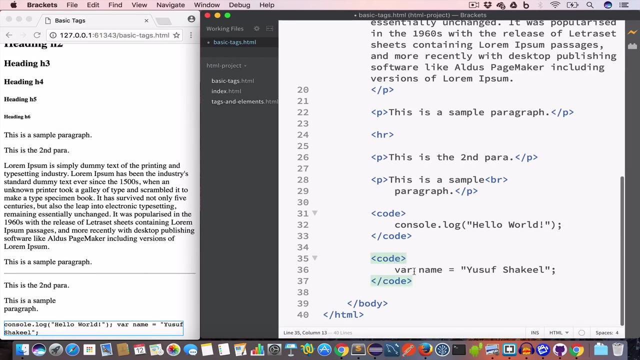 And similarly we can also show another code And let's say, this time we are going to write Hello world Say: var name equal to Yusuf Shakeel. So you can see, the code tag is not a block element. So the next code that we have written, var name equal to Yusuf Shakeel- it starts right. 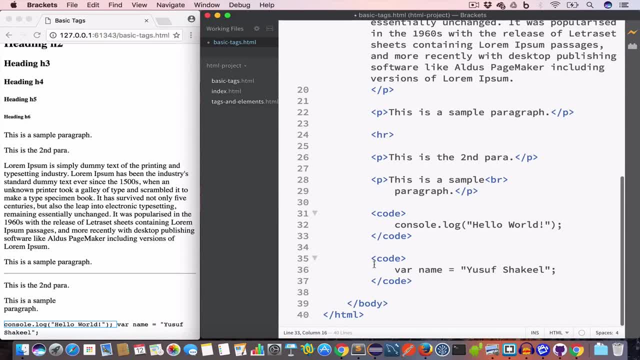 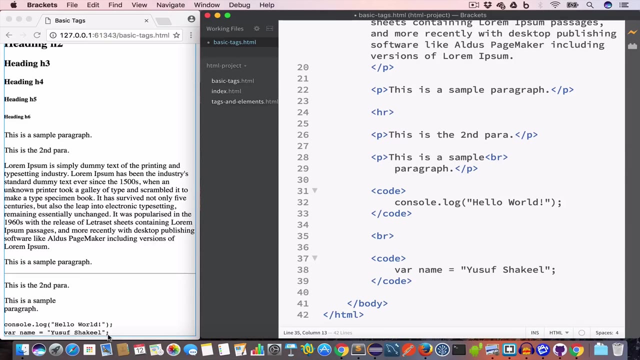 after the first code. So in order to bring the second code element, That is, the opening code tag, the content and the closing code tag- After this first code element, we'll use the BR tag. Now you can see: the first line of code and the second line of code are now in a separate. 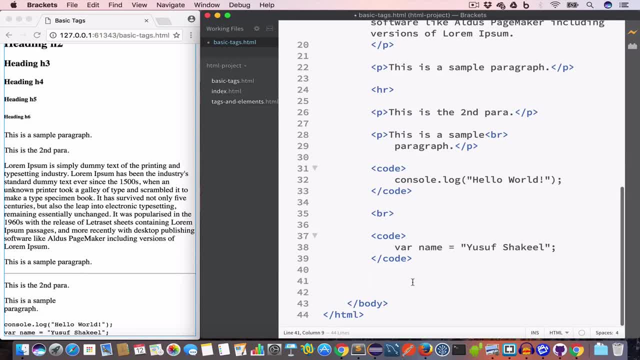 line. The next tag is the pre tag or pre formatted tag, And this is the first line of code And this is the second line of code. And this is the first line of code And this is the second line of code. It is used to preserve the formatting of the document. 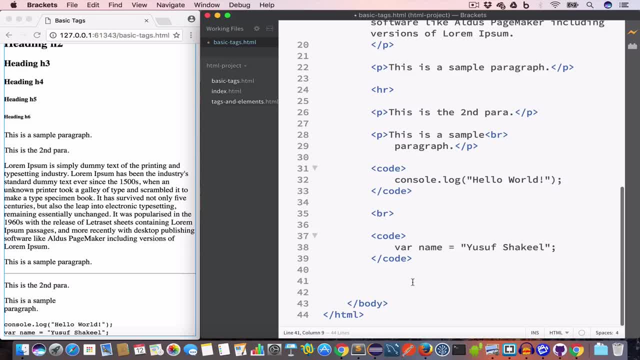 Now, as I mentioned earlier, even if we create multiple spaces between two words or we give multiple new line between two words, HTML will still consider them as one character. For example, if we create a paragraph and we write this, you can see the output. 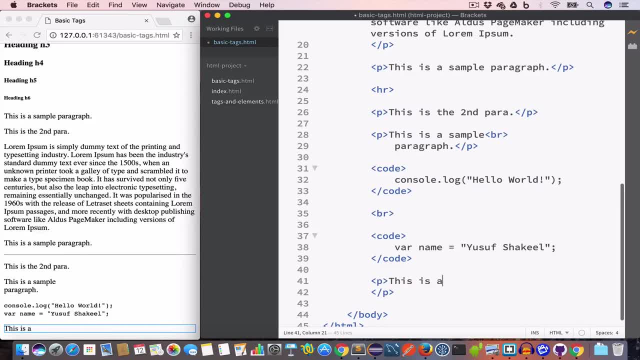 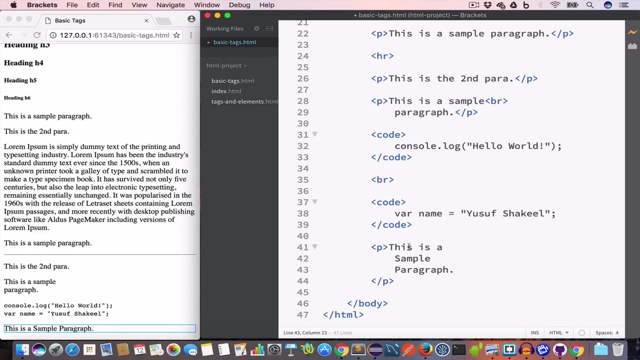 This, This: This Is a Sample, Sample paragraph, So we have written: this is a sample paragraph in three lines, But you can see the output is in a single line. So in order to preserve the formatting, This These: 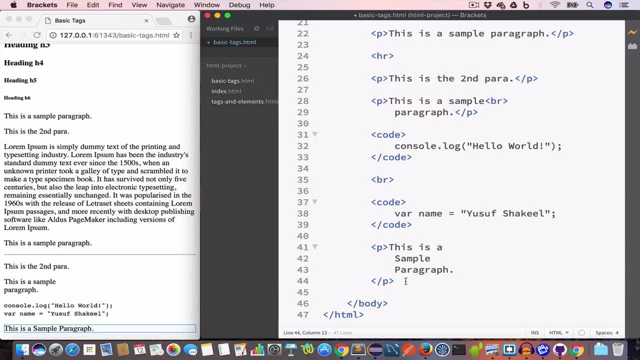 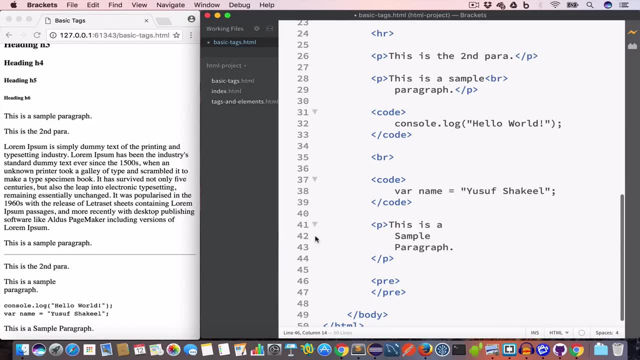 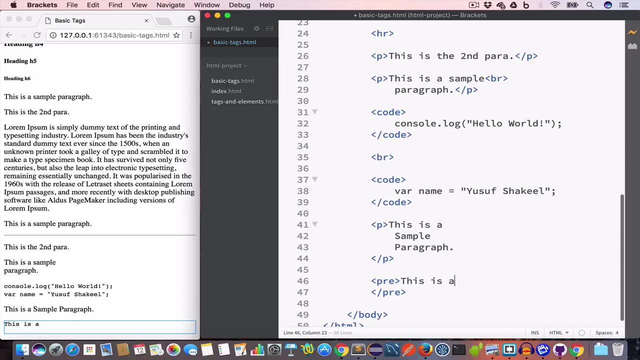 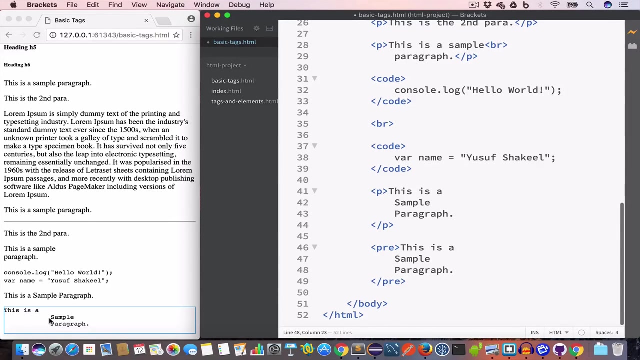 we use the pre tag. so let me go ahead and create a pre tag and this time, if we write this is a sample paragraph. Now we can see the output is in three separate lines and the sample word is having multiple white spaces before it. This is because the pre tag 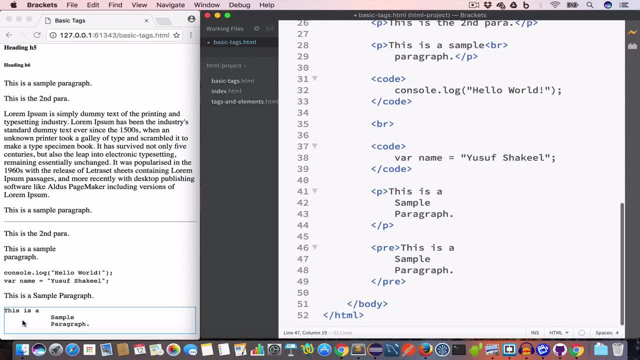 is preserving this white spaces in the output. So in order to make this sample word, this one, start from the very beginning of the line, we have to remove the white spaces before it. Similarly for the word paragraph. now, if you look at the output, we can see this is a sample. 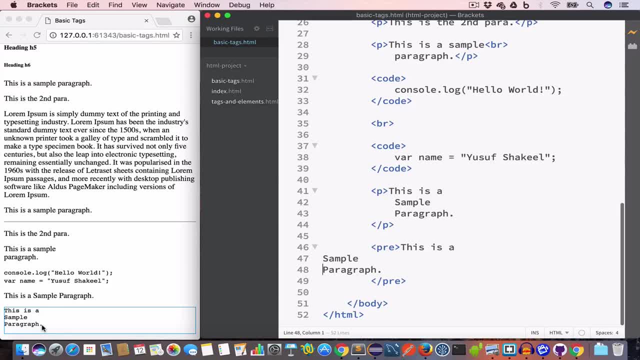 paragraph. the output in three lines and each starting from the very left, without any white spaces before the words, and if you look at the last line you can see we have an empty line. This is because the word paragraph ends at the third line. but before the closing pre. 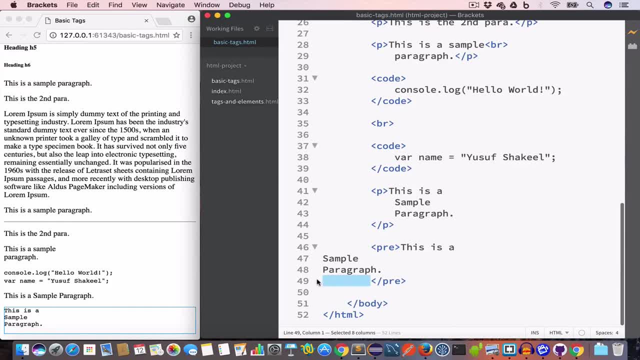 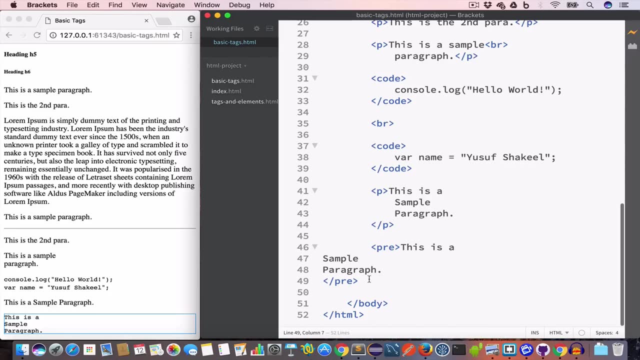 tag, we have this fourth line, which consists of white spaces. So in order to remove this fourth line, we have to remove this white spaces. The next tag that I want to talk about is the anchor tag, or the a tag. It is used to create hyperlinks in the website. 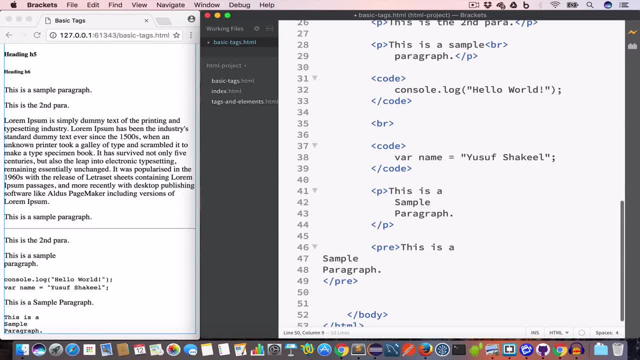 So, for example, if you want to create a link to DY classroom from this basic tags dot HTML file, We can write dyclassroomcom and we can give this anchor tag an attribute href, and then we can set the href value to https: wwwdyclassroomcom. 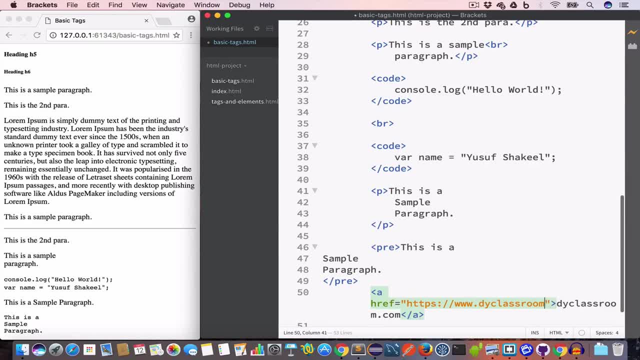 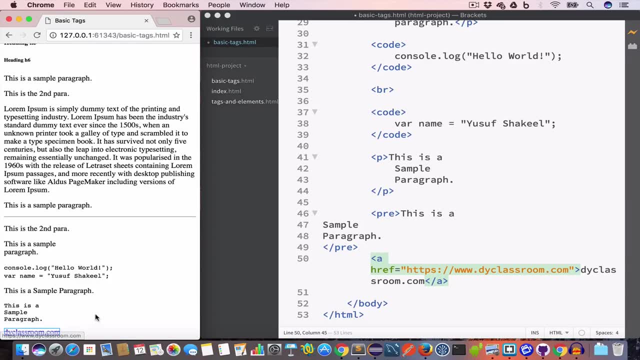 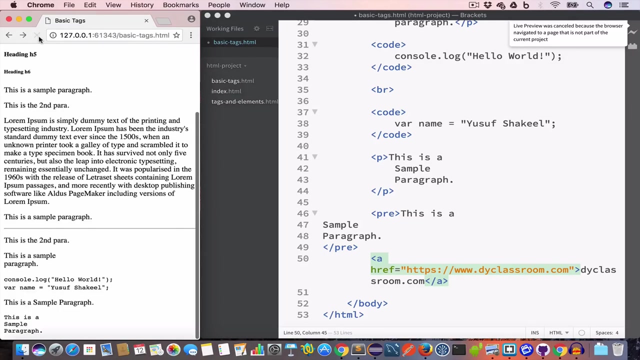 Okay, Thank you, Bye, Bye, Bye, Bye, Bye, Bye. So you can see, we have this link, or the anchor tag, and it is pointing at the classroom website. So if we click on this, it will take us to the DY classroom website. 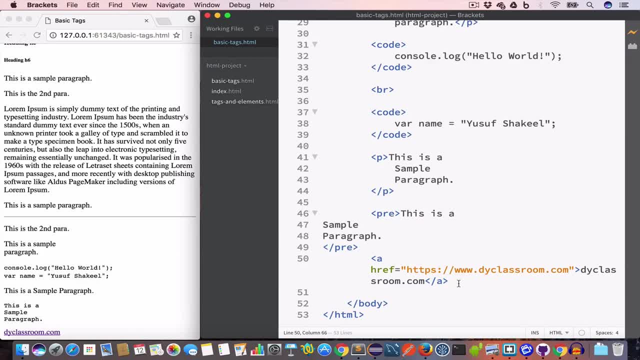 And now let us talk about the image tag or the IMG tag. So, in order to show image, we use the image tag. so in this example, let me go ahead and create an image tag and this image tag takes an attribute- SRC- and the value of SRC. 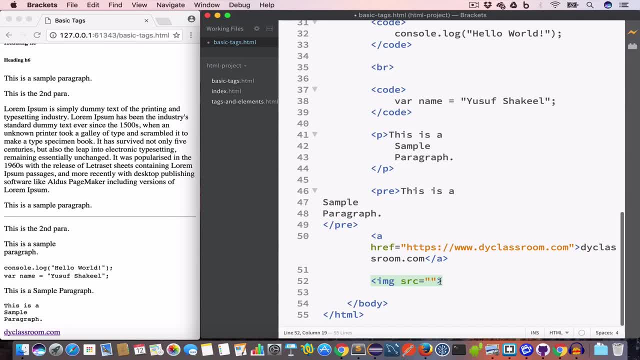 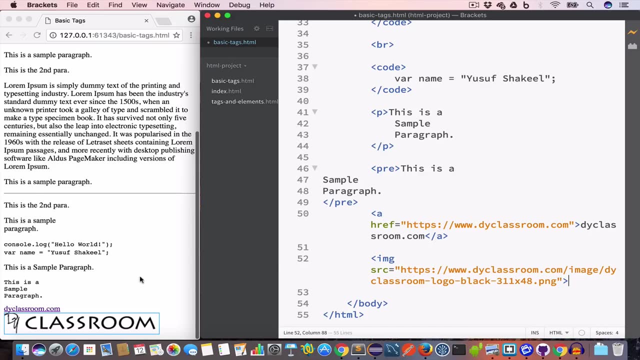 attribute is equal to the path of the image file. in this case, I'm going to set the SRC value to DUI classroom logo, so I'll paste the link of DUI classroom image and now, if you see the output, you can see the logo of DUI classroom website. now, an interesting thing that we can do with an anchor tag and image tag. 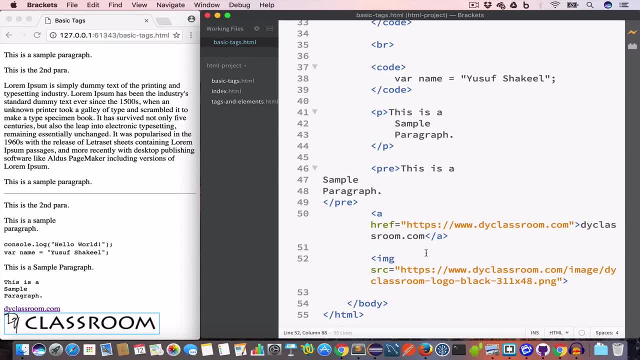 is to create a clickable image, a hyperlink image, that is, an image which will take the image tag and paste it in the image tag- and paste it in the image tag as well when we click on a button or if we click on some screen in my Charleston. 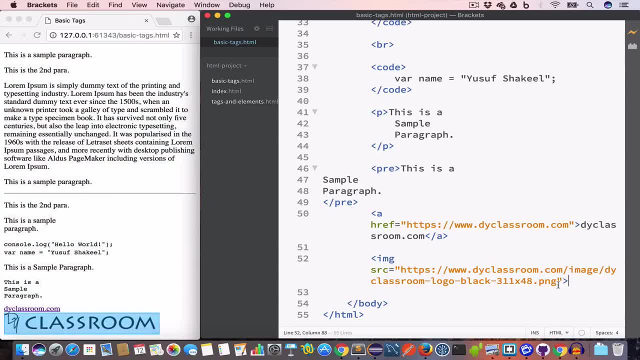 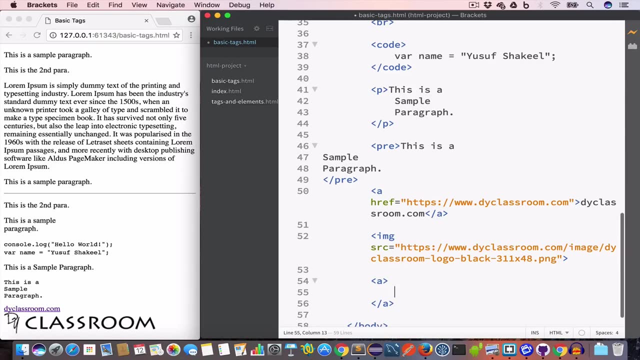 える page. this tag is going to take us to some other website or another page when clicked. now, if we look at this image tag, it is just a simple image and nothing happens when we click on it. now, in order to create a hyperlink image, all we have to do is create an anchor tag and inside the anchor we create an. 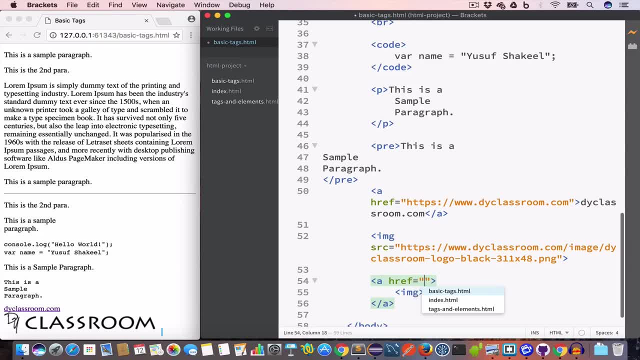 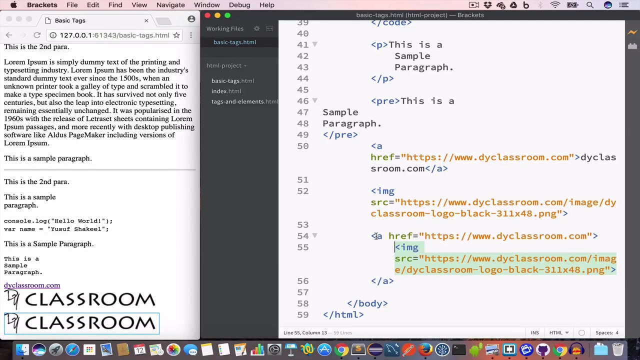 image tag and of the anchor tag to the url where we want to redirect, in this case dyclassroomcom, and we set the image src to the image we want to use, in this case the logo of dy classroom. so now you can see we have an image tag inside an anchor tag. so 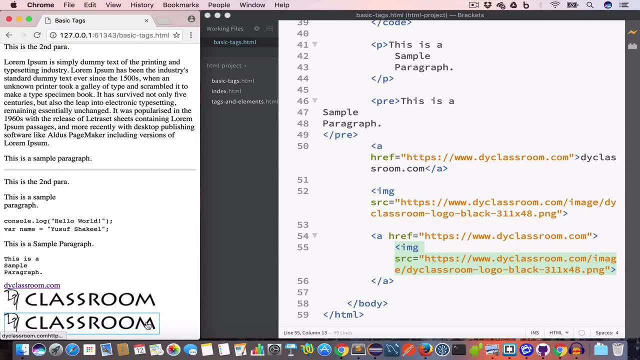 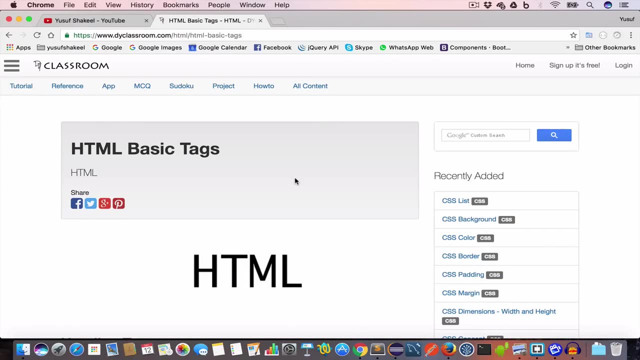 this image is now clickable. it is now a hyperlink image and when we click on it, it will take us to dyclassroomcom, like. so all right guys. this brings us to the end of this tutorial. i hope you will find this video interesting and, if you do, please give this. 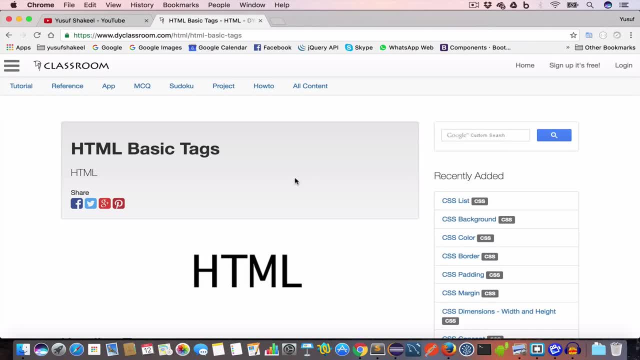 video a like and please subscribe my channel because i make new videos every week and, guys, i'll put the important links in the description below. the notes of this tutorial is on my website, dyclassroomcom. the link will be in the description and the code that we are writing in this tutorial series. i'll put them in my github repository.